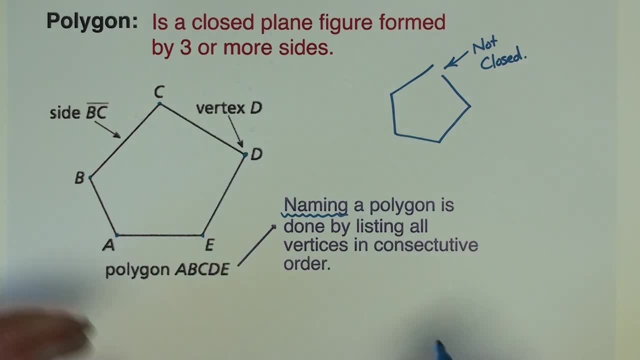 all of the vertices that make up the polygon. So if I were to draw a figure like this, all the vertices, okay, And I get to list the vertices in consecutive order. So this particular polygon has five vertices. so we just simply name it polygon and you can go in either direction. 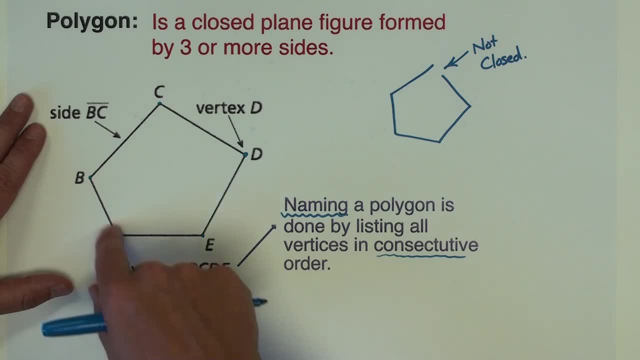 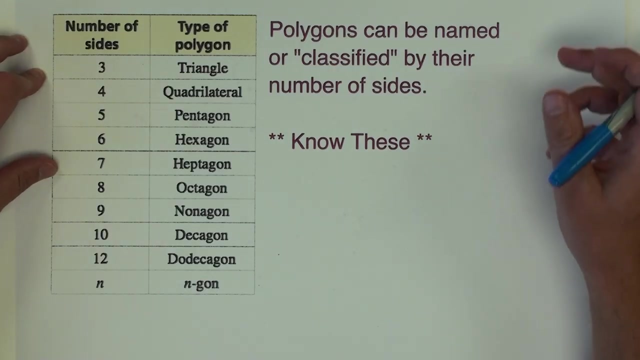 but here it's polygon A, B, C to E, so A to B to C, to D to E. You can start at any point and you just need to go around the polygon in one direction, listing out every single point. Now, this particular slide has some information on it that I no doubt believe that you're aware of. 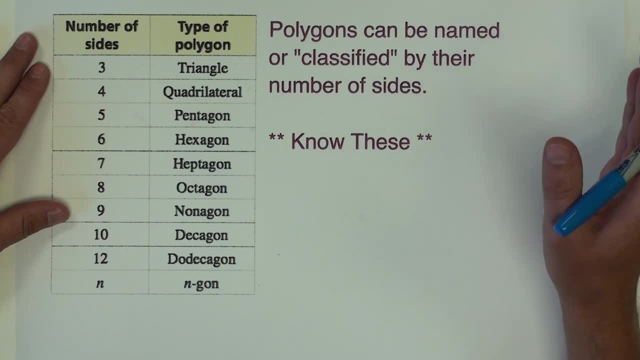 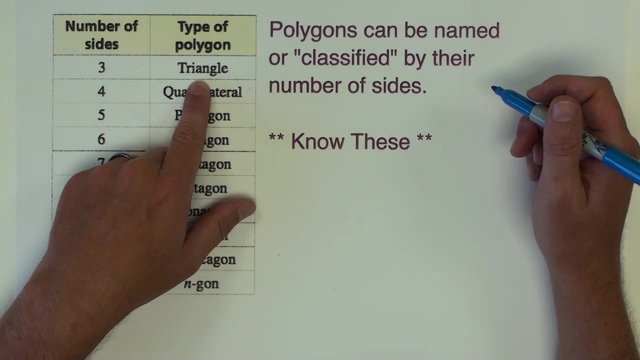 you've at least heard as you've gone through your grade levels up to this geometry course. But polygons can be classified by their number of sides And like these names, no doubt you've heard some of them. Like, I'm sure everybody knows what a triangle is. Triangle, if I ask you to draw. 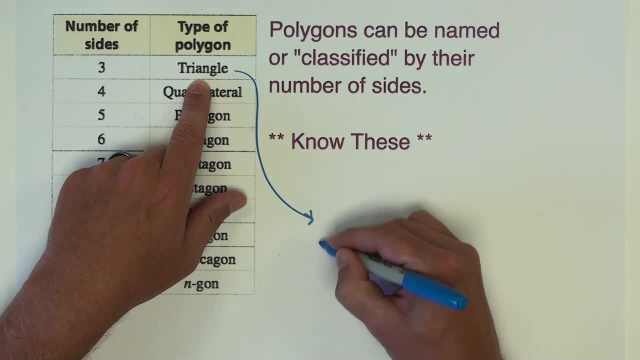 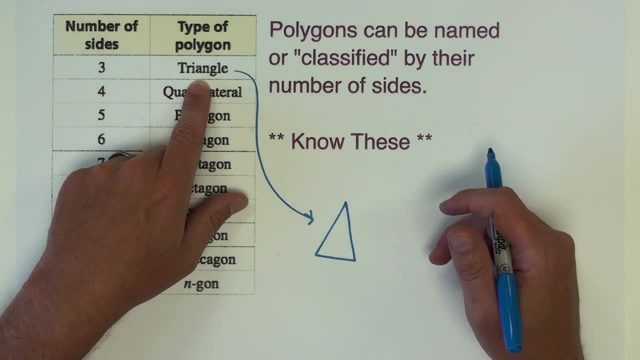 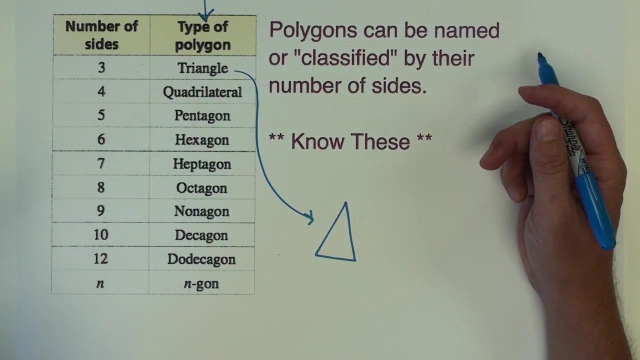 a triangle, right? We'd all know what a triangle is. So if I were to draw a triangle, I'd ask you to just draw something like that, right? We know what these shapes are going to look like. What you need to know are the names of these, okay? So there's not really much that I need to write on. 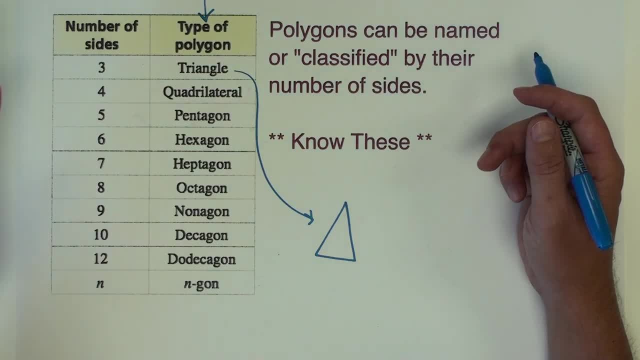 this slide. It's just something that I think you should hit pause. take a moment to read through these, The ones that you don't know. maybe make note of that. maybe jot them down in your notes. work on memorizing the names. 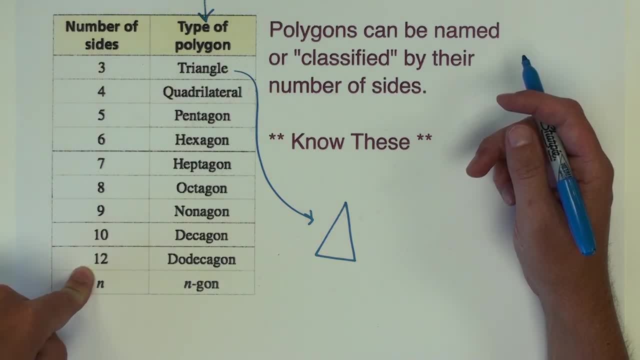 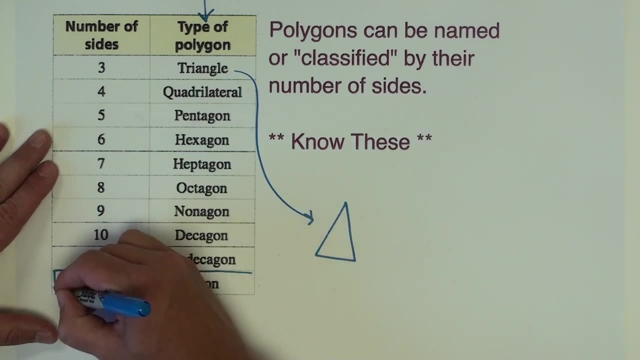 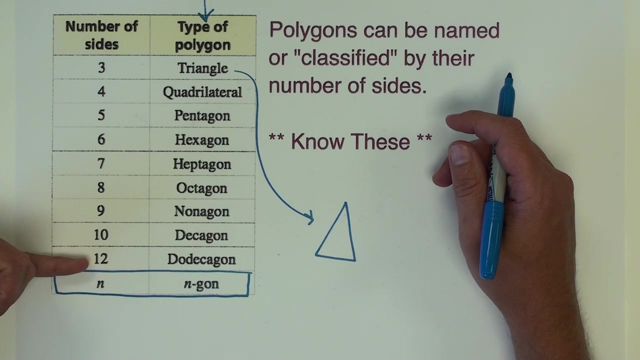 What are the names of these different polygons and how many sides polygons have. Now one note here, the bottom line in this table. there are names for polygons beyond 12 sides. Nobody needs to really memorize those names. If you needed it, you could certainly just look it up. So if there's 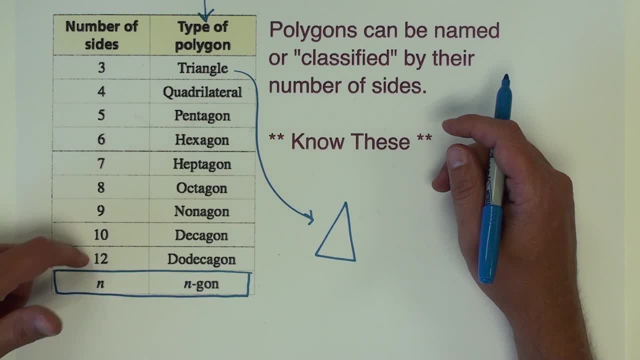 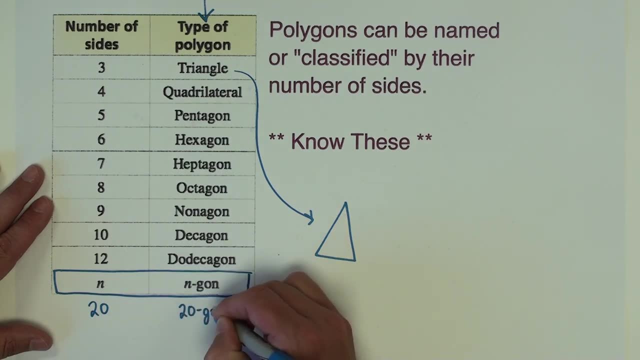 a polygon that is more than 12 sides. let's say we have a polygon with a number of sides, with 20 sides, we would just simply call it a 20-gon, So you can do that kind of naming system for anything larger than 12.. Now all polygons are going to fall into one of two. 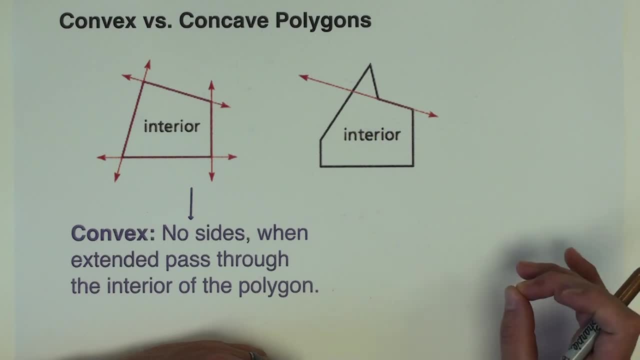 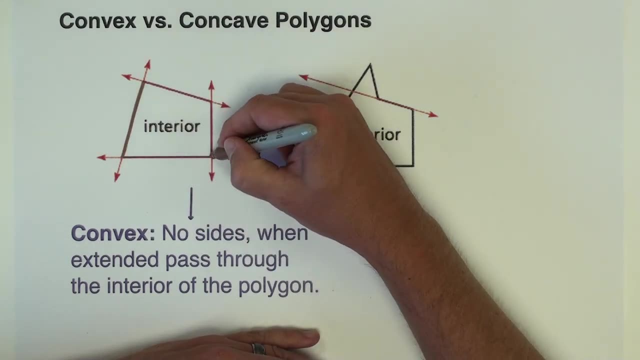 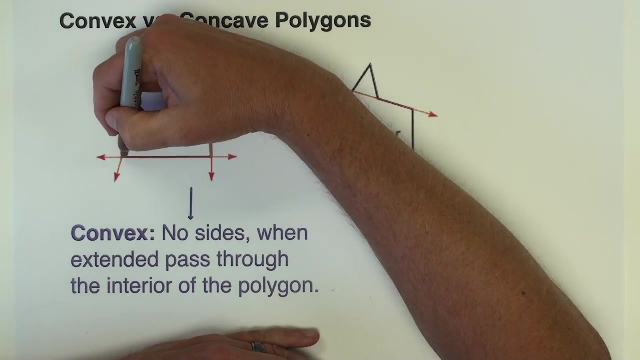 categories. They're either going to be what we call convex or concave. So I want to look at this polygon here. I'm going to trace it out and then we'll look at the definition here. So here's the actual polygon. It's a four-sided polygon, So this is a quadrilateral and a convex. 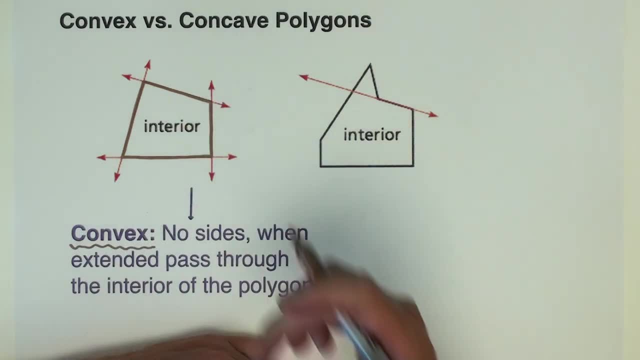 polygon, which is what I just traced out right here. The definition of convex is that no sides- okay, so none of the sides of the polygon, when extended, are going to pass through the interior of the polygon. okay, So you see that. 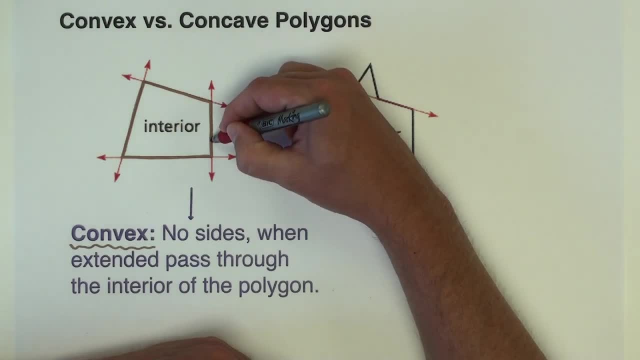 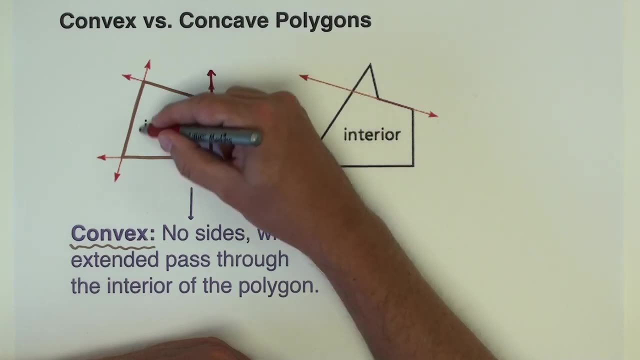 With the red lines already. so like this side right here, if I take this side and extend it here and here, notice it didn't pass through the inside. okay, It stayed on the outside of the figure. Well, all the sides, when extended, don't pass through the inside. And because 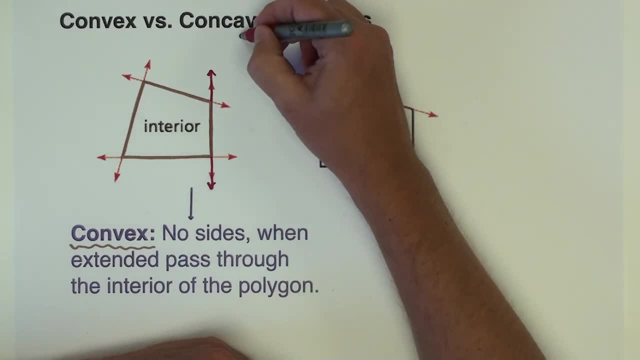 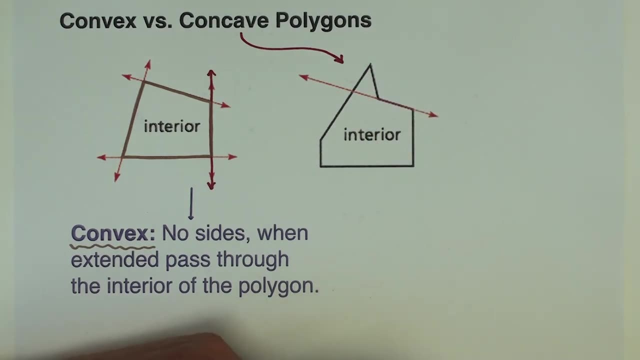 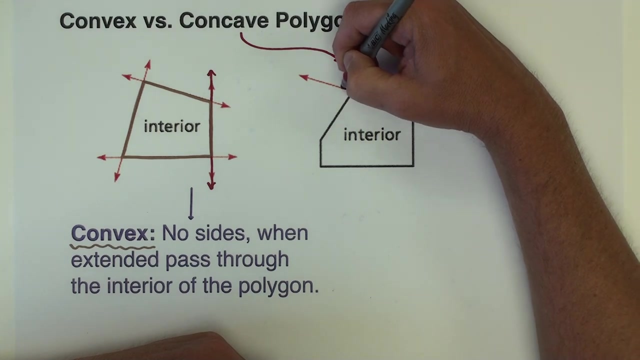 of that that makes it convex. Now, on the other hand, a concave polygon, all right. So let's take- I'm not going to trace the whole thing, but let's look at this side right there. Well, if I take that side and I extend it here and here, notice that it does pass. 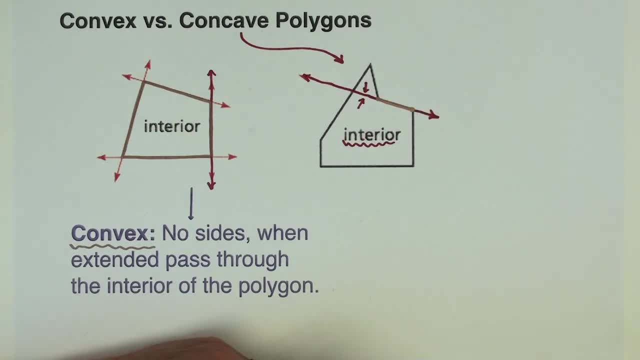 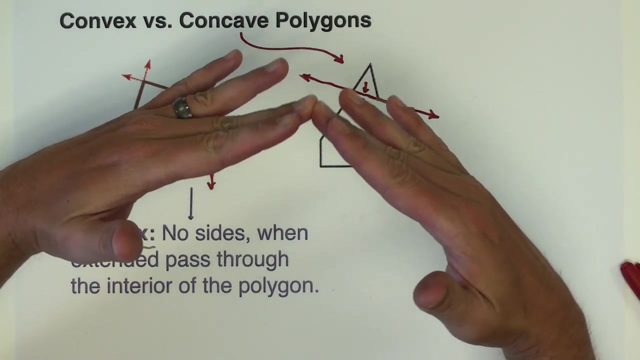 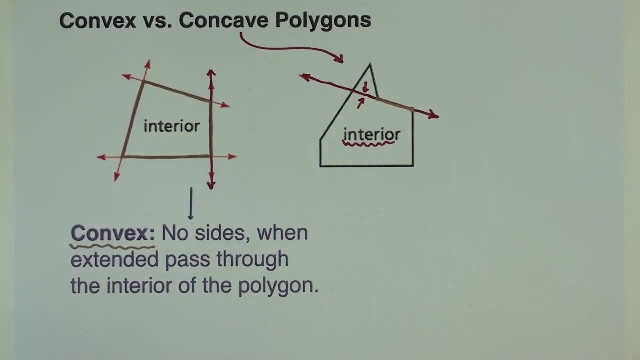 through the interior of that polygon And because the extended side passes through, we can't classify it as convex. We're going to classify it as concave, okay. I kind of think of this as like if the shape caves in on itself, that's a concave polygon, okay. So let's look at an example where we 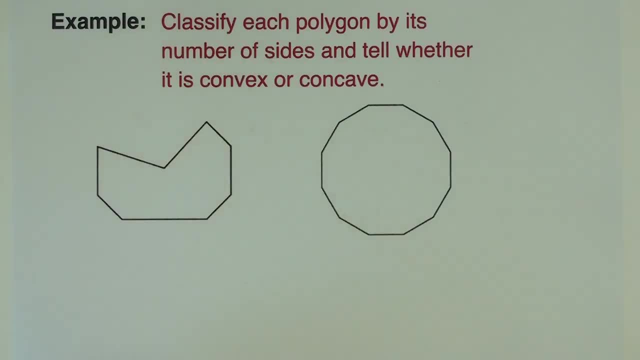 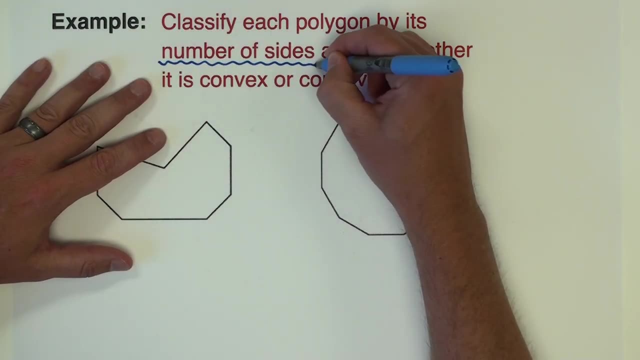 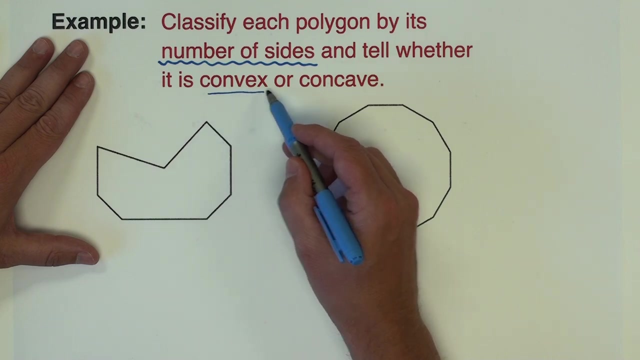 practice classifying the difference between these two. Okay, the directions on this slide ask us to classify each polygon by its number of sides. okay, So that's the chart from a few slides ago, And then tell whether it is convex or concave. okay, So two things we're trying to do here. 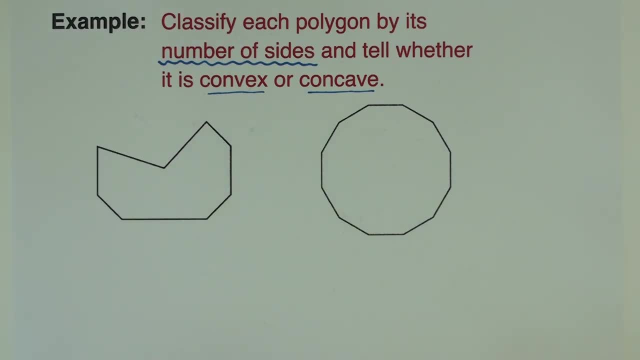 What's its name? by how many sides it has, and then is it convex or concave. So let's start on this first one on the left. Let's just count the sides One, two, three, four, five, six, seven, eight. There are eight sides in this polygon. If it's eight sides, then 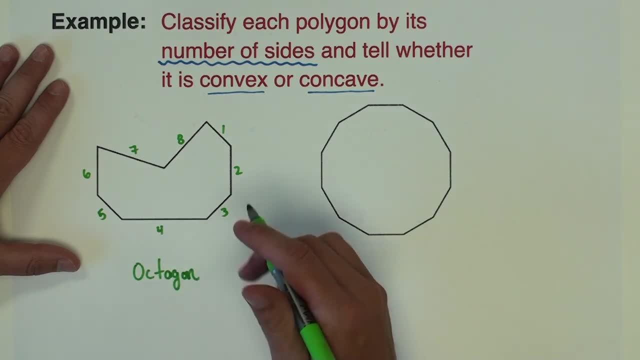 we have an octagon. Now this side right here of this octagon, when extended notice, it passes through the inside. That means this is a concave octagon. Now other example to the right. let's name it first by its number of sides. I'm going. 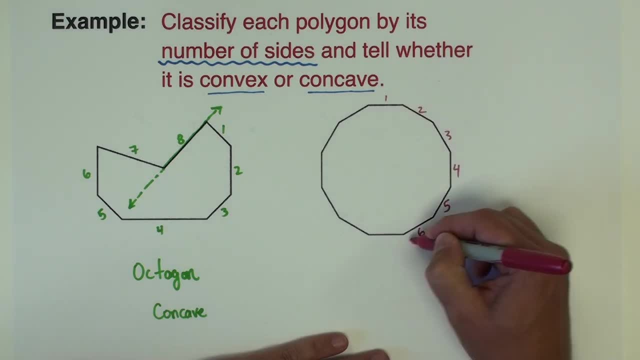 to number them, just to make sure I don't miss any. Sometimes, when you count, once you get around to the inside, you hit the left, you hit the right. This is a concave octagon. Let's start on this one on the left. Let's just count the sides One, two, three, four, five. 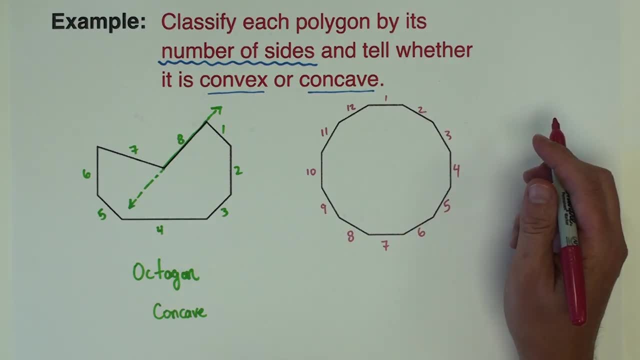 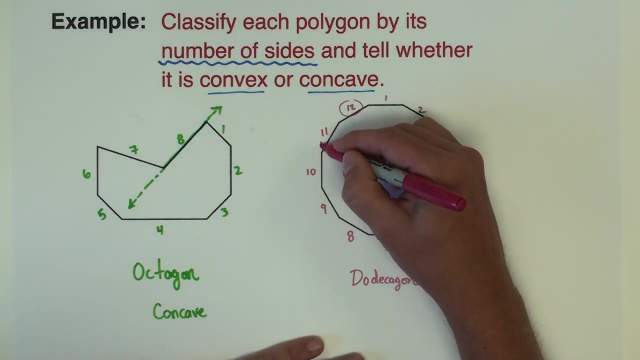 And you might find that you've forgotten where you started. So I find numbering them is pretty easy to prevent that from happening. But I have 12 sides- 12 sides is a dodecagon- And notice that any of these sides that I pick, like this one right here, doesn't pass inside. 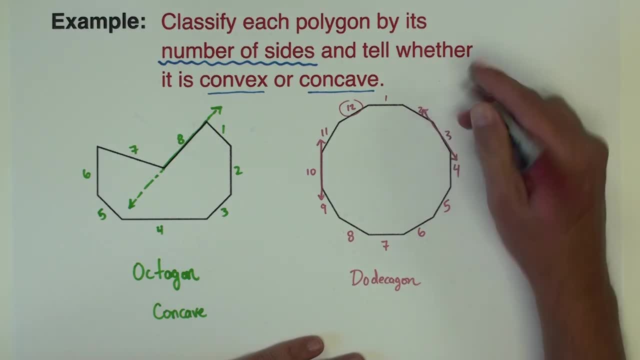 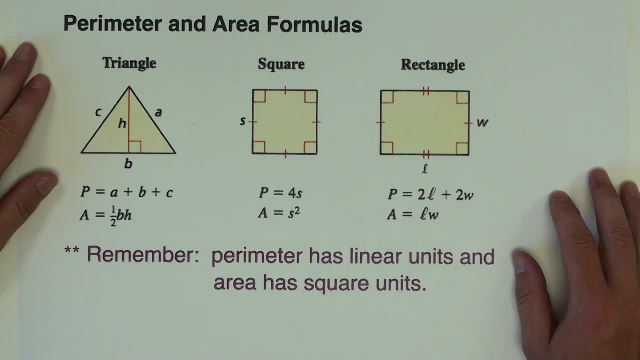 This one over here doesn't pass inside. None of the lines extended are going to pass inside. It makes that convex. Okay, now we're going to do something that should be familiar to, hopefully, everybody watching this video. If you've made it to a point in your life where you're taking a course in geometry, 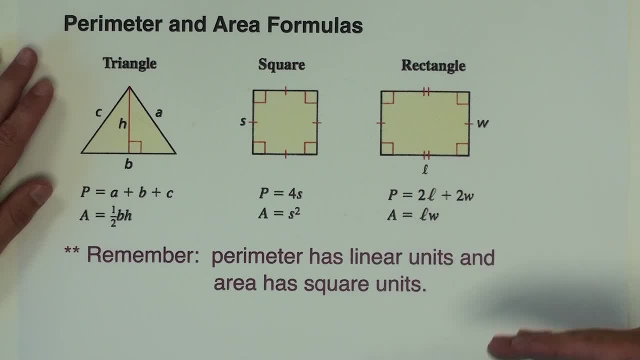 you've no doubt had some geometry lessons kind of along the way in your other math classes, And one of the things you're definitely going to see along the way is perimeter and area formulas, And so we're just going to do a few shapes in this particular lesson today. 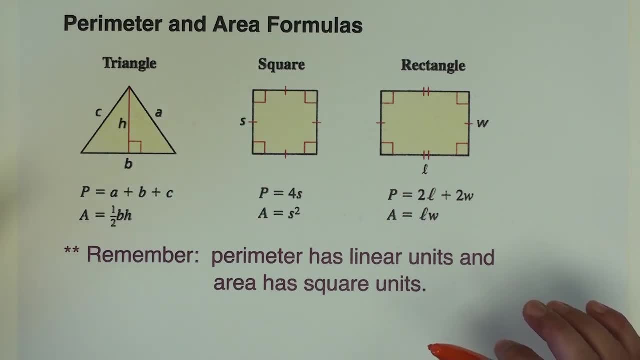 Throughout Throughout the course. we do a lot more of this kind of later on, But for now, just triangles, squares and rectangles is what we're going to look at. It's what we're going to see in the assignment for this lesson. 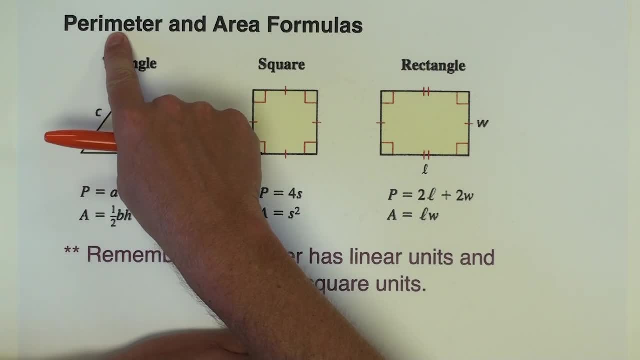 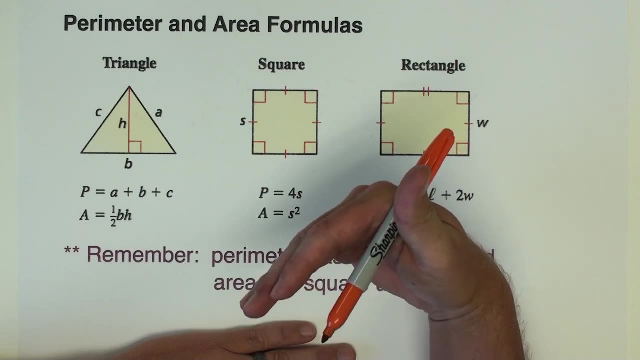 So, first of all, remember that perimeter is just simply the distance around the shape. You really don't need formulas for that, because all you're doing- like right here, all you're doing- is adding three sides together. Or here in the square, you're adding s plus s plus s plus s, or four times s, all right. 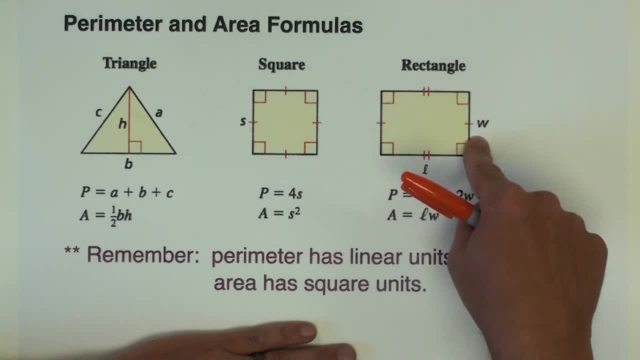 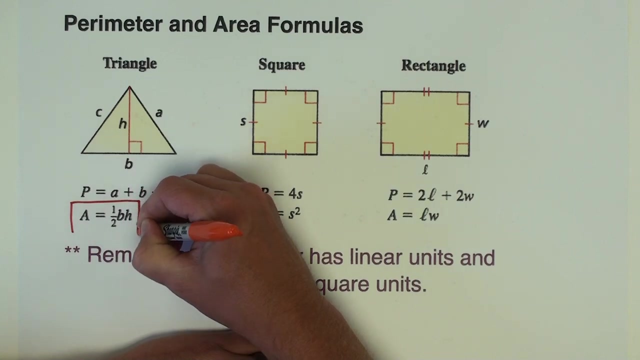 Or here you're adding length and length and width and width. You can work them as formulas, but really it's just add all the sides up. That's. perimeter Area is a little bit trickier and we do have some formulas, so I do recommend that you memorize these formulas. 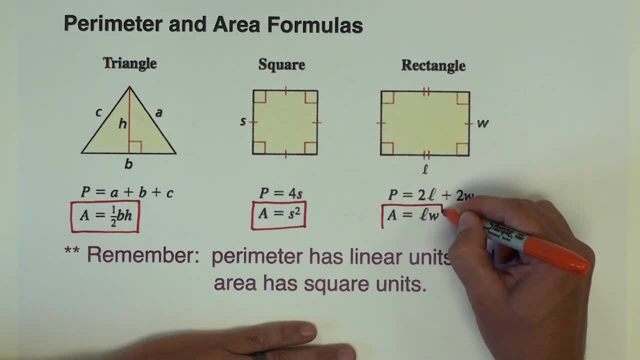 And we'll do examples, And we'll do examples that are going to show these as well. But again, you've certainly seen these, so we're just kind of reviewing this. Area of a triangle is half its base times its height. Area of a square is its side times, side or side squared. 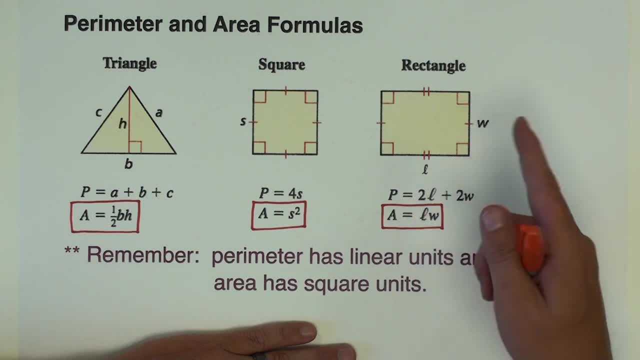 And area of a rectangle is its length times its width, which is kind of like square. It's also side times side, but the sides can be different. so length and width, Sometimes people do base and height Of rectangles as well. As long as you kind of know the idea of how to do it, you can memorize the formulas if you want. 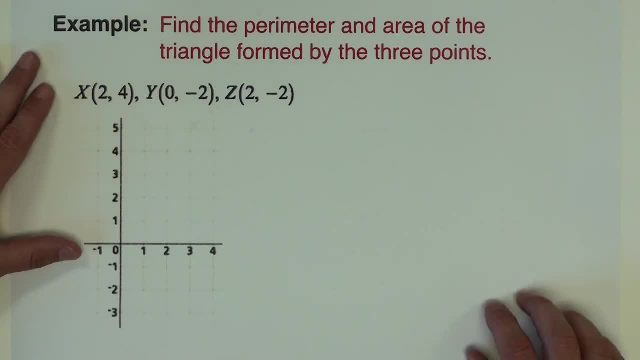 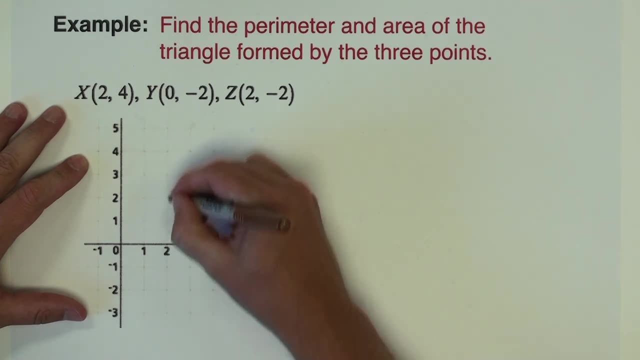 All right, let's look at some example problems. Okay, find the perimeter and area of the triangle formed by the three points. So let's plot it out first. So point x is at 2, 4. Point y is at 0, negative 2.. 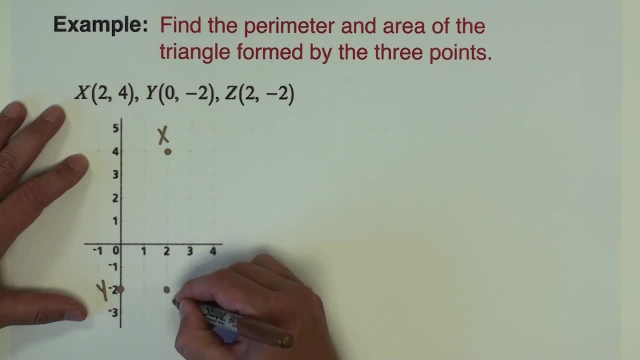 And z is at 2, negative 2.. So I've got this triangle right there. Now, as far as perimeter goes, I need to find all the lengths. I'm just going to count this out, at least the ones that I can. 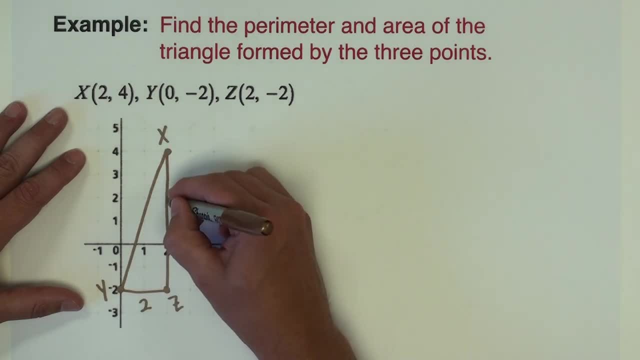 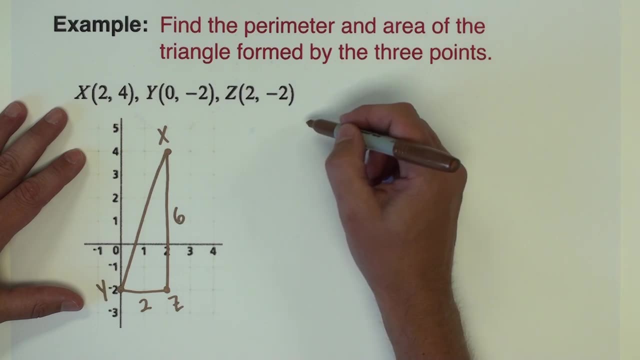 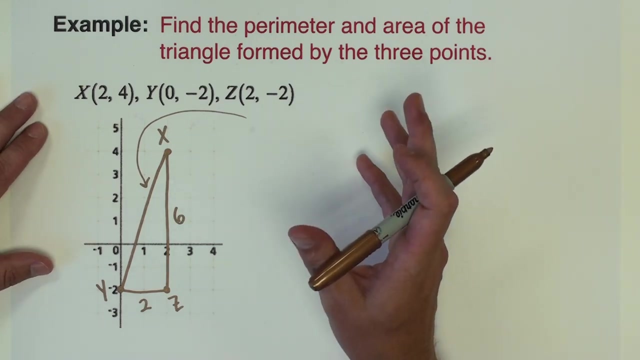 yz is 2,, xz is 1,, 2,, 3,, 4,, 5, 6.. To find the perimeter I'm going to have to know the length of this side Right here. So this is like a distance problem. 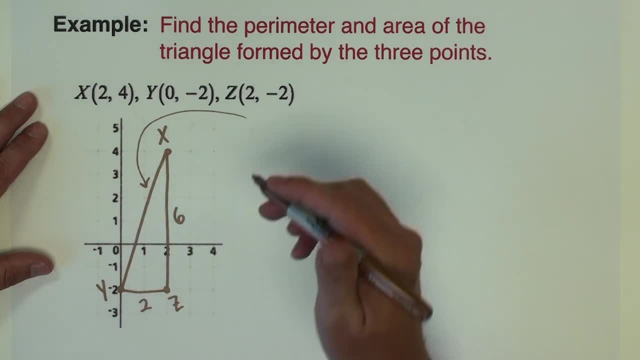 What's the distance between points x and y? I can find the difference or the distance by doing Pythagorean's Theorem. I can do 2 squared plus 6 squared equals c squared. So I've got 4 plus 36 equals c squared, which is 40, equals c squared. 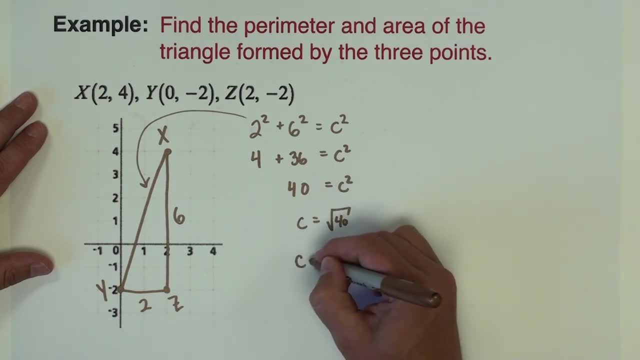 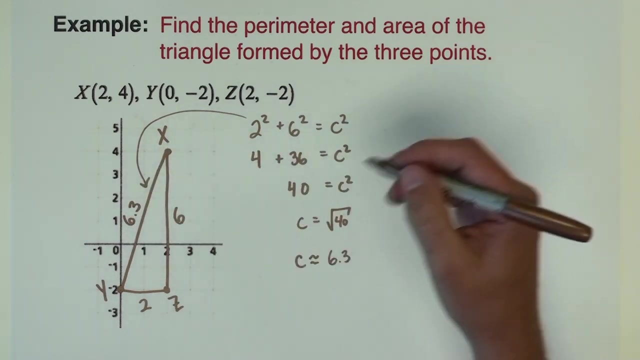 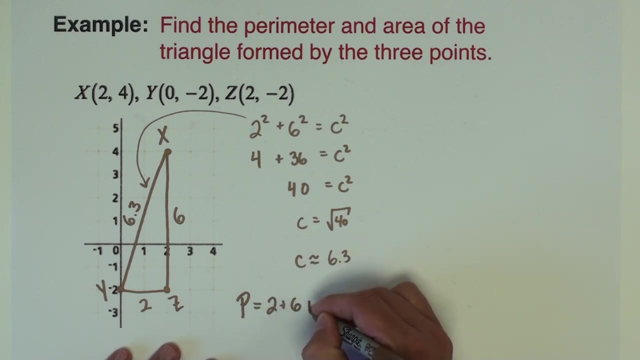 So c is the square root Of 40.. And the square root of 40, let me get my calculator out- The square root of 40 is about 6.3.. So that's the length, right here. So our perimeter- then let's do p for perimeter- is going to be 2 plus 6 plus 6.3.. 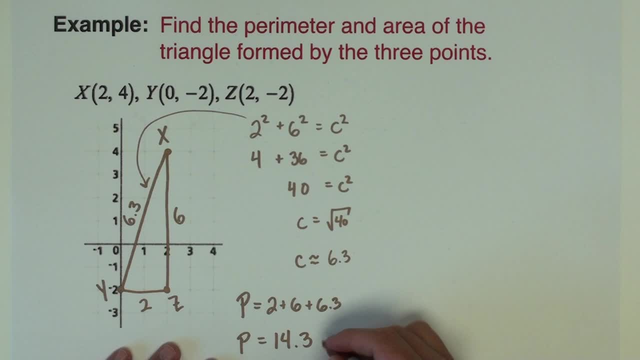 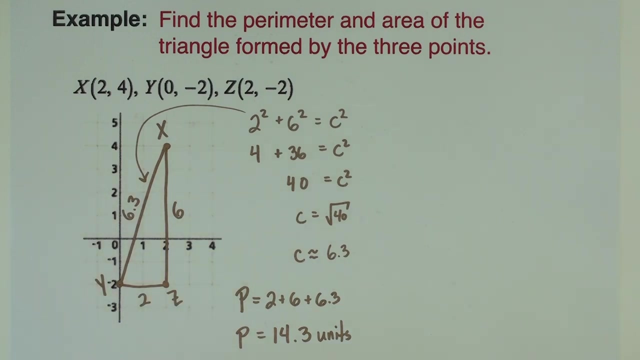 The perimeter looks to be 14.3.. I'm going to put units, Okay. Hopefully we can see that on the video. Okay, next let's do area Now for this particular triangle area is going to be much, much easier to find. 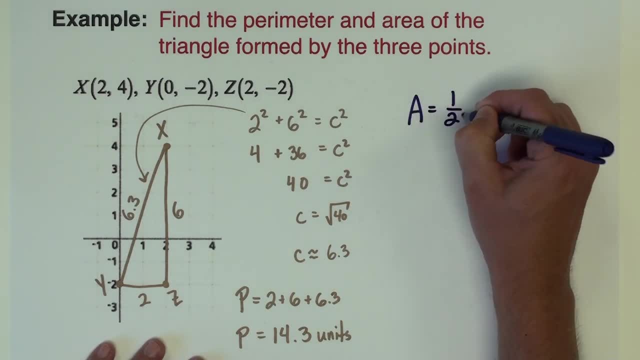 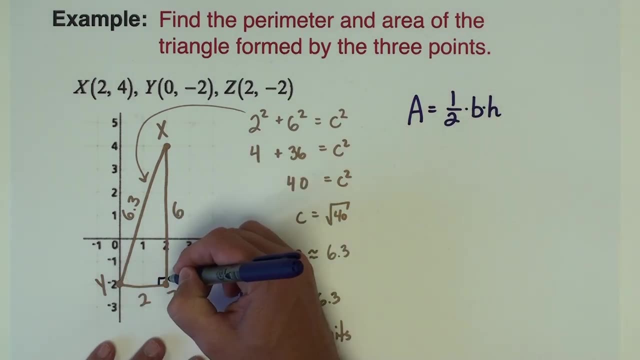 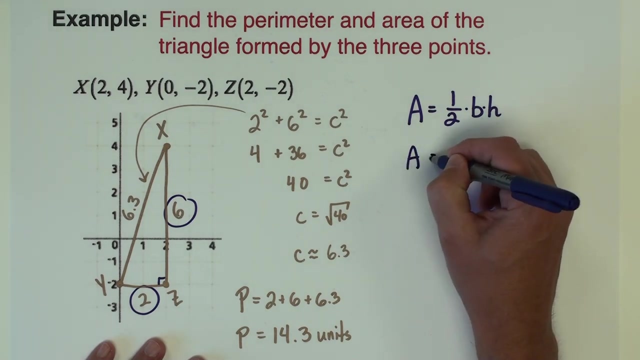 Much less. work Area of a triangle is half times its base, times its height. Now, this triangle that we have is a right triangle. The base and the height are the measurements where the right angle meets. So, in any order, half times 2 times 6,, 2 times 6 is 12, and half of 12 is 6.. 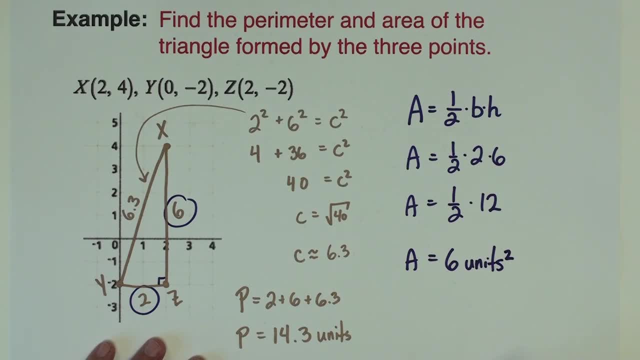 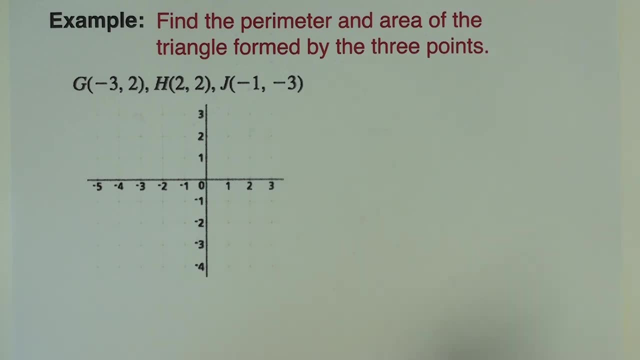 Because this is area we want the units to be squared. Okay, this next problem. I have another triangle, So, if you want, you can certainly pause this, work it on your own and then press play to check your work, But I'm going to go ahead and get started on it. 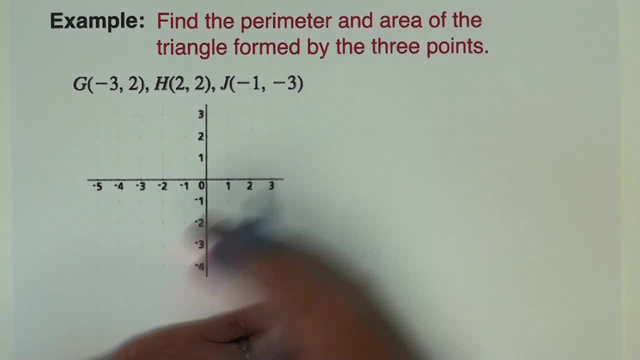 Right now. you can take notes on it if you want Or, like I said, just try and work it yourself to see if you've got it down. So the triangle is at the negative 3, 2.. It's a point G. 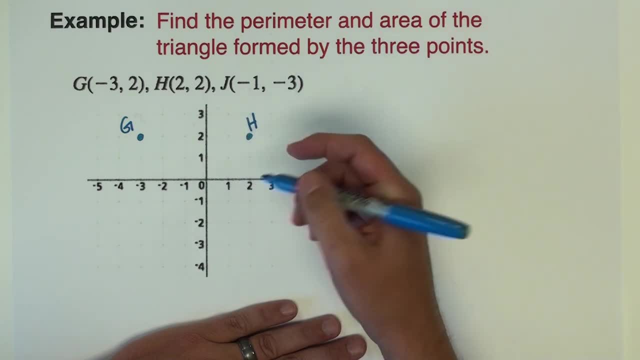 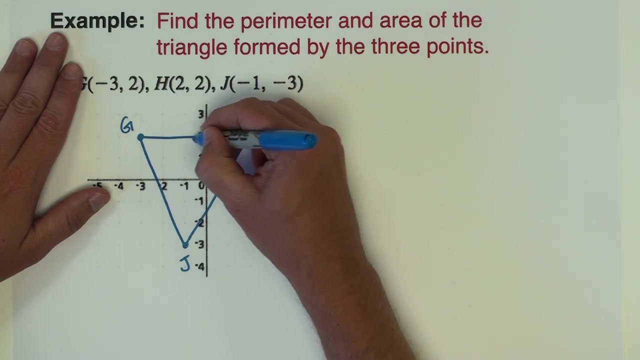 2,, 2, point H, Negative 1,, negative 3, point J, And so like this. Alright, so perimeter: Define the lengths of all the sides. Now GH, right, here is the easy one. I can just count that out. 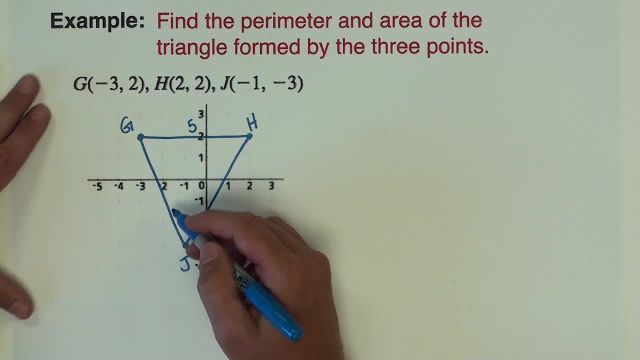 That's 5 units. To find GJ, however, I'm going to have to do Pythagorean's theorem, So let's see To get from G to J. I'm going down 5.. I'm going over 2.. 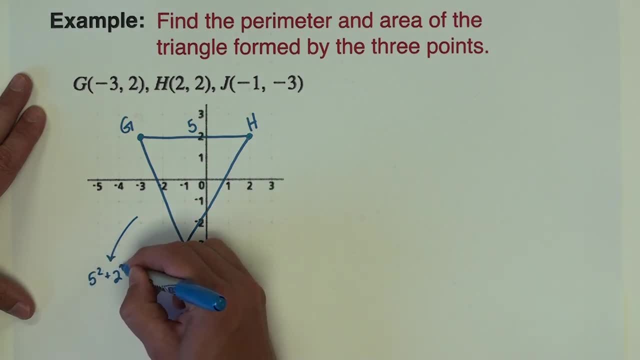 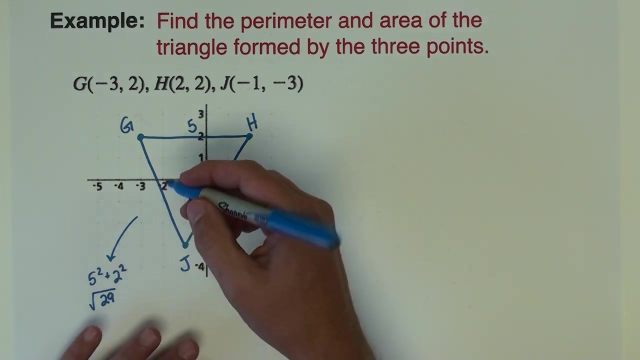 So this is going to be 5 squared plus 2 squared, That's 25 and 4, which is 29.. So I want the square root of that, And the square root of 29 is about 5.4.. And over here for HJ, I'll do the same thing. 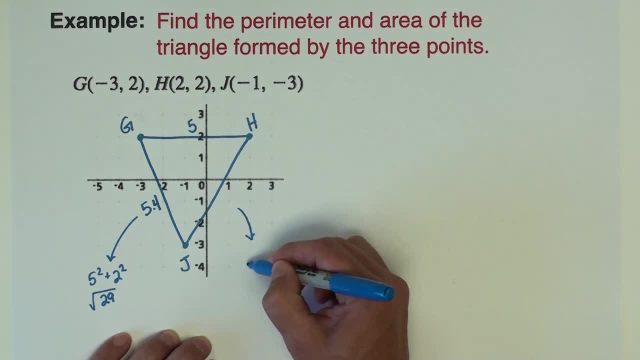 From H to J. it's down 5., But it's over 1,, 2,, 3. So that's 25.. And 9. So that's 34.. I want the square root of that 34., Which is about 5.8.. 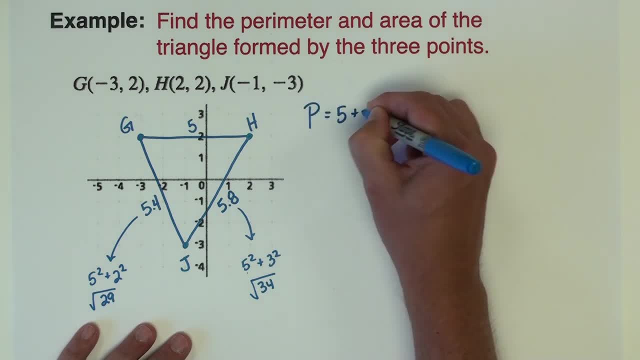 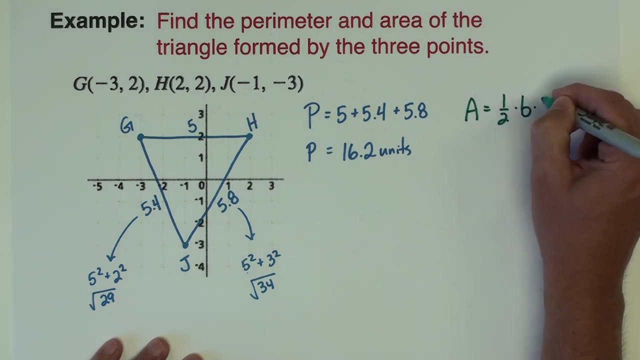 So the perimeter then is going to be 5 plus 5.4 plus 5.8.. So I get 16.2 units. Now to find the area For area I need to do again the formula as half times base times height. 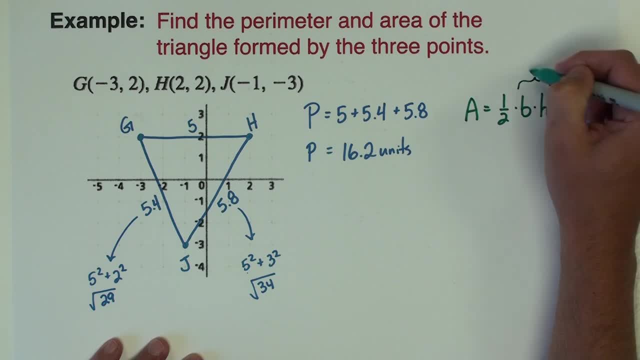 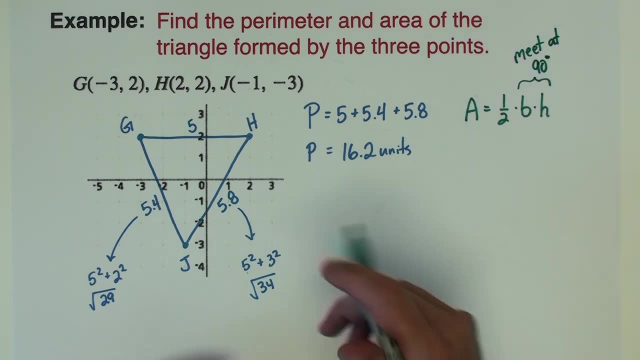 Remember, the base and the height meet at a 90 degree angle, And so, if I look at all these angles, none of those are right angles. I know what right angles are, even though we haven't talked really about angles yet. I know what 90 degrees looks like. 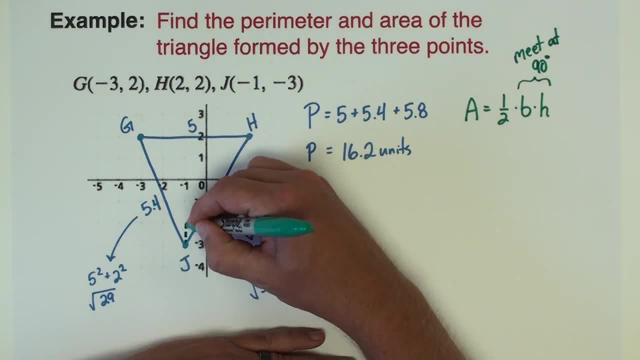 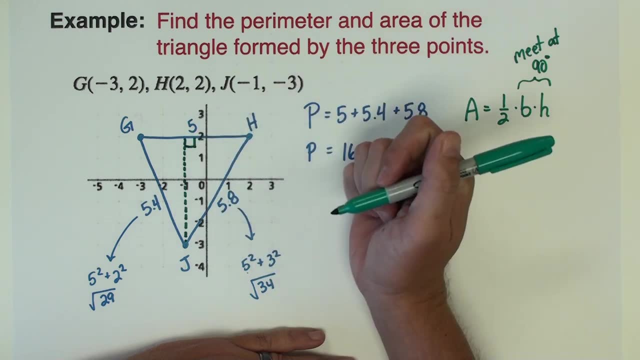 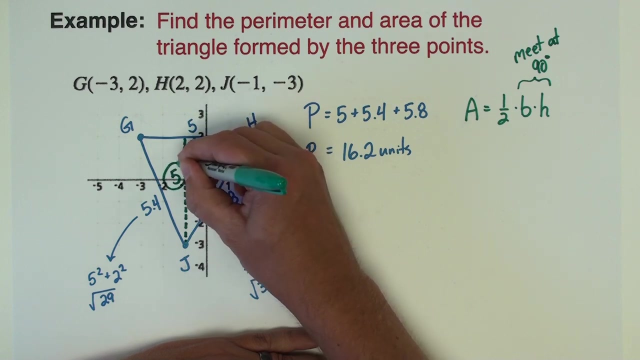 So I have to create a 90 degree angle. I can come straight up from point J to that segment and make a 90 degree angle, And that is 1, 2, 3,, 4, 5.. So my base and my height are these two segments, and they're 5 and 5.. 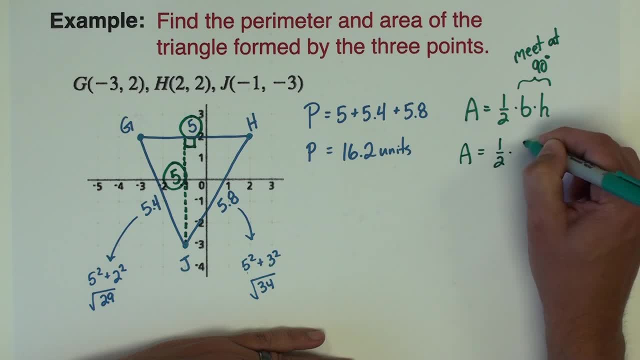 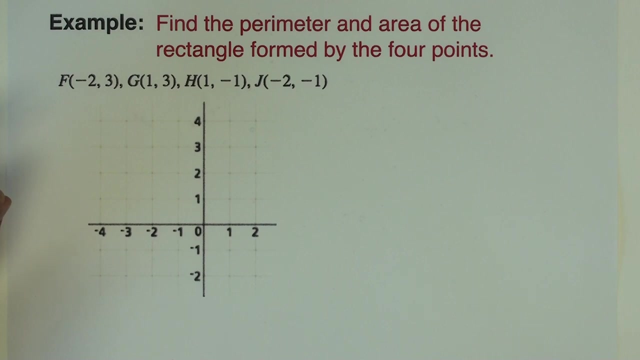 So my area is half 5 times 5.. 5 times 5 is 25.. And half of 25 is 12.5.. Area has square units. Okay, next one. we're going to find the perimeter and area of the rectangle formed by the four points. 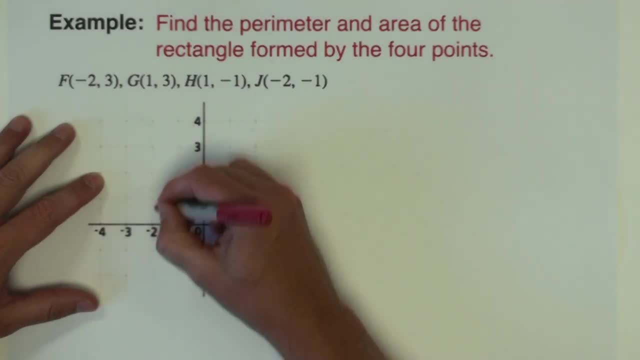 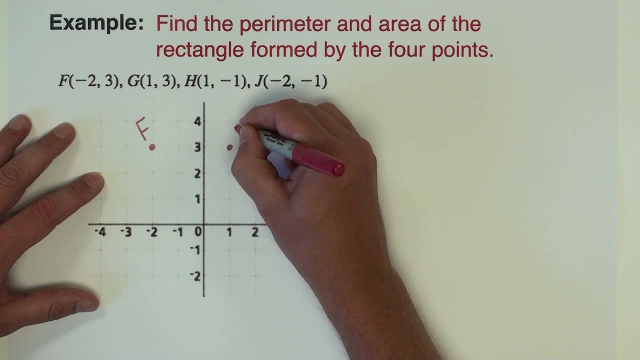 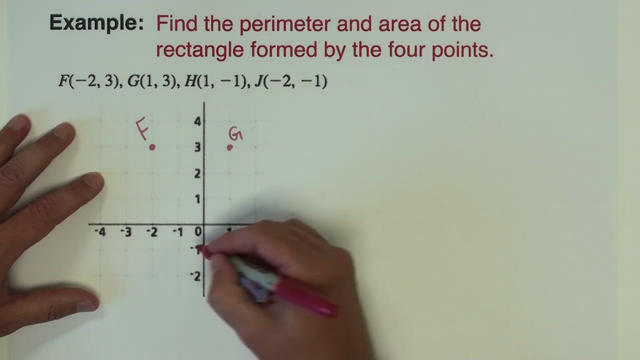 So let's plot this out. to begin: F is at negative 2, 3.. G is at 1, 3.. I is at 1, negative 1.. Sorry, H is at 1, negative 1.. And J is at negative 2, negative 1.. 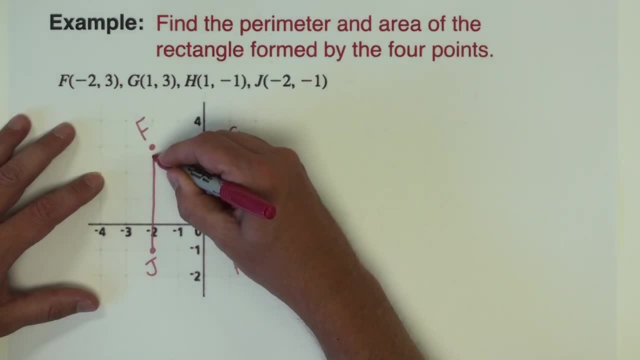 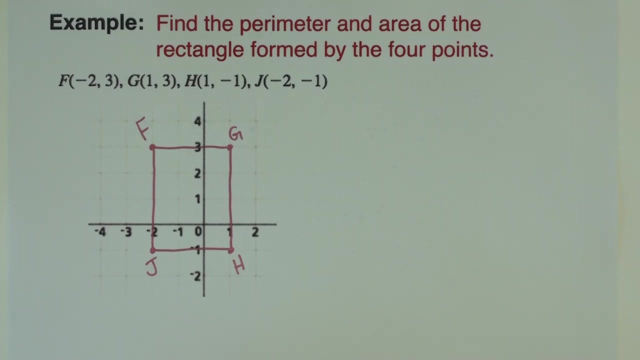 So here's four points that are the vertices of a rectangle. Okay, so let's start with perimeter. Perimeter is the distance around, So from F to G is 3.. G to H is 4.. J to H is also 3.. 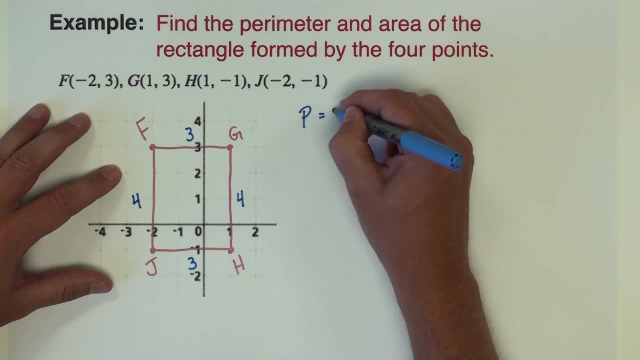 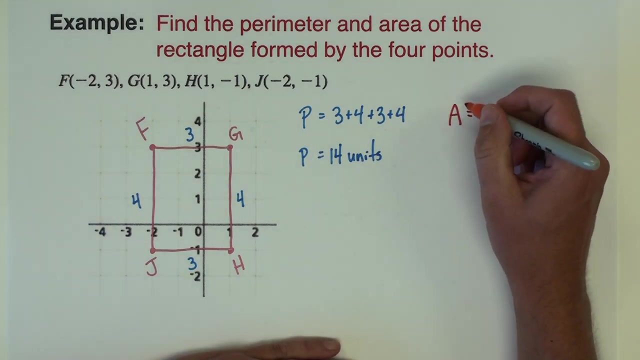 This is also 4.. So the perimeter is going to be 3 plus 4 plus 3 plus 4, which is 14 units. The area can be done two different ways. You could just count how many squares are inside that rectangle, certainly. 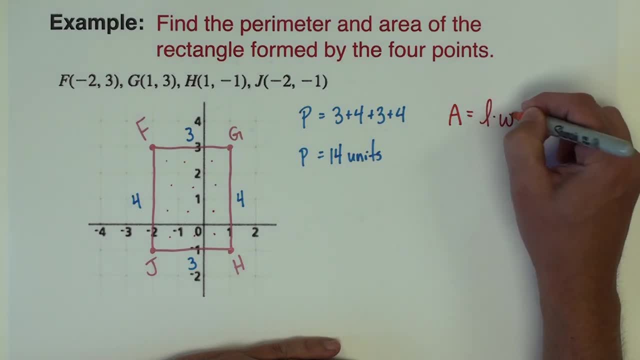 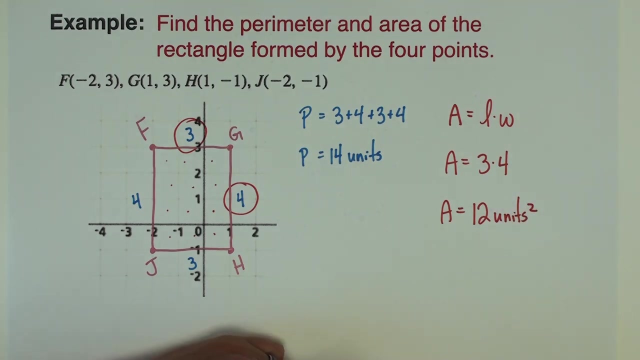 Or you can do this, Or you can do the length times the width. The length times the width are the two different dimensions there. So area is going to be 3 times 4, which is 12 units squared. Okay, we have one final example. 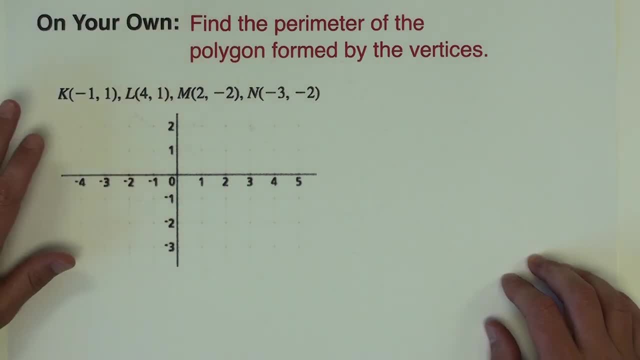 The directions say: on your own. So you can certainly pause this and work it out on your own if you would like, And then unpause it to see what the answer is at the end, Or you can follow along. I'll leave that up to you. 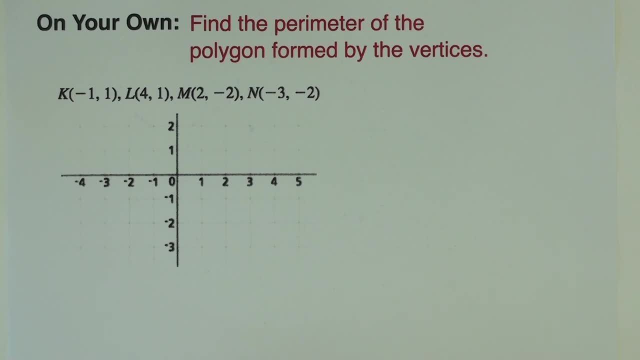 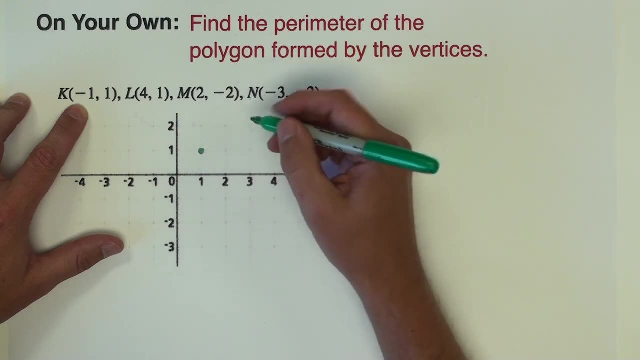 But we want to find the perimeter- It's just perimeter- of the polygon formed by the vertices. So let's begin by plotting this out. So we've got a point at negative 1, 1.. We've got a point at 4, 1.. 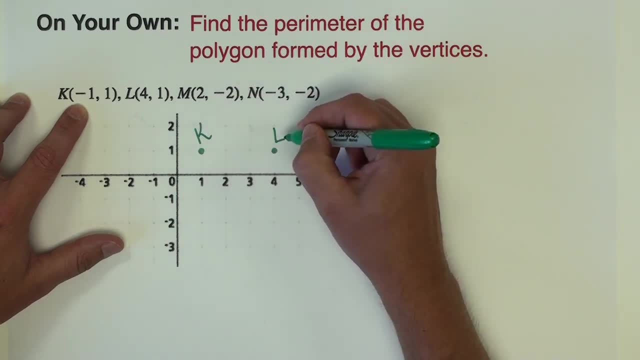 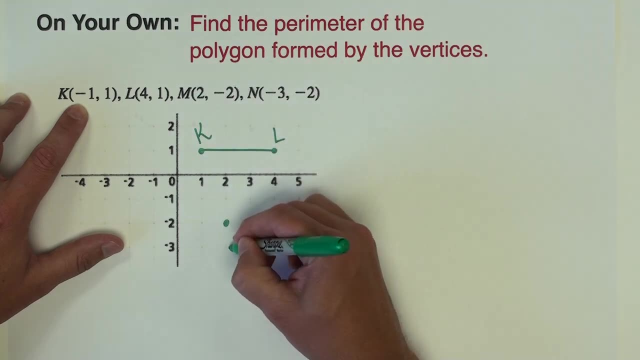 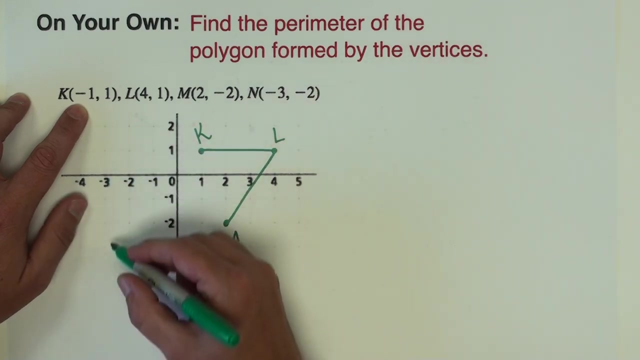 Let's go ahead and label these two. That's K, That's L. We've got a point at 2, negative 2.. That's M. We have a point at negative 3, negative 2.. That is N. 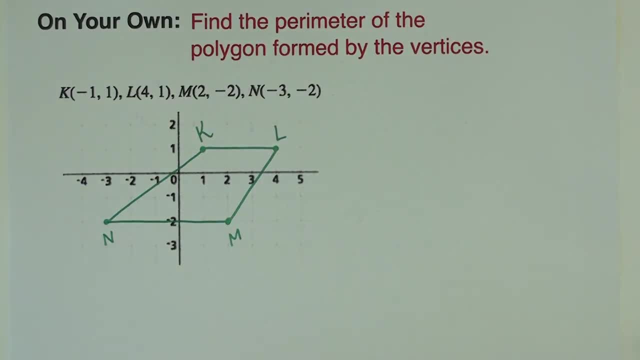 Okay. so to find the perimeter I need the lengths of all four sides. I'm going to start with the easy ones. From K to L, I can count, That's 3.. From M to N: 1,, 2,, 3,, 4,, 5.. 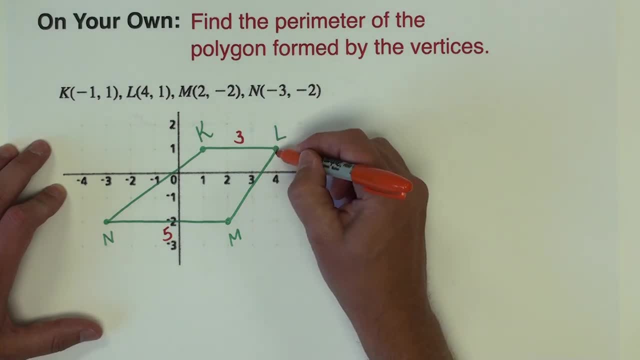 Okay, those are the easy ones. Now for the other two, for ML, I'm going to have to see this as a triangle, which is 2 by 3.. So the length of ML is going to be the square root of 2 squared plus 3 squared. 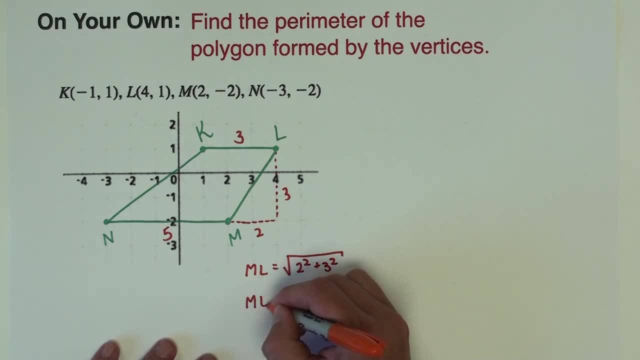 That's coming straight from Pythagorean's theorem. So ML is the square root of 4 and 9, which is 13.. The square root of 13,. we've seen that already in a separate problem. The square root of 13 is about 3.6.. 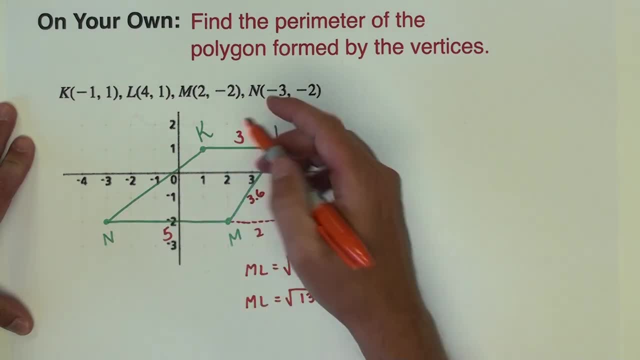 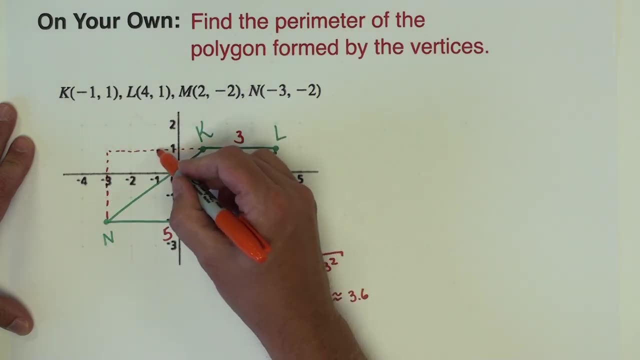 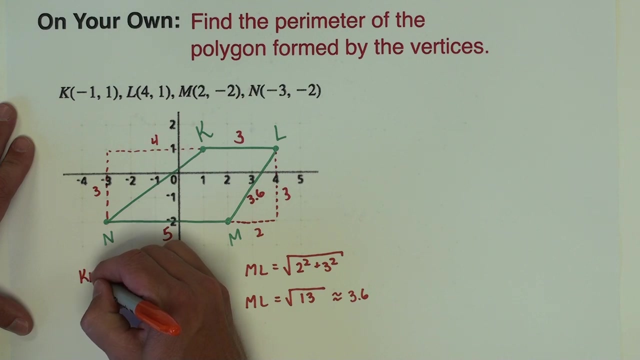 I need to do the same thing for KN. So KN that triangle is 1, 2, 3, 4, and 1, 2, 3.. So KN From Pythagorean's theorem is the square root of 3 squared plus 4 squared. 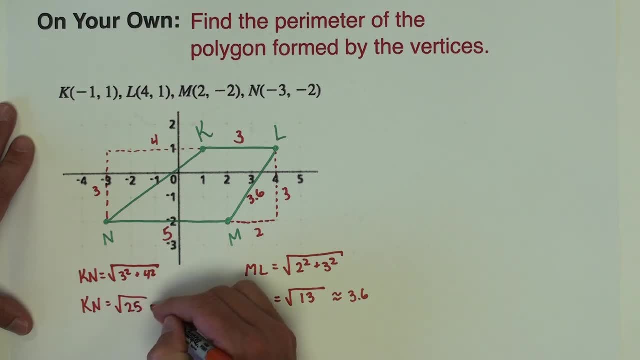 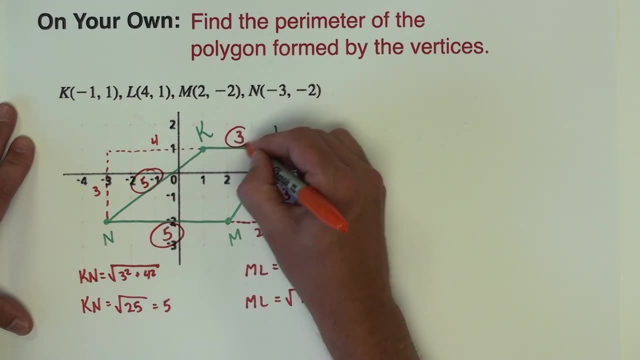 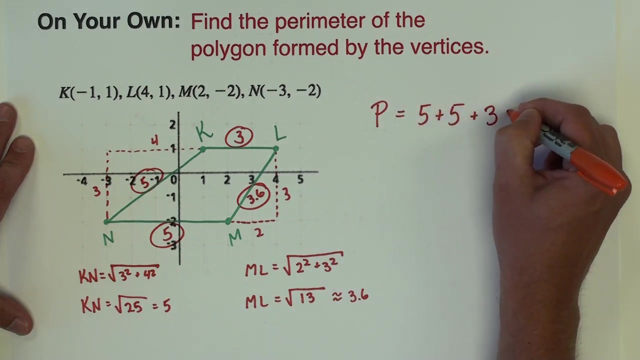 That's 9 and 16,, which is 25,, which is 5.. Okay, so our four sides are 5,, 5,, 3, and 3.6.. So the perimeter is 5 plus 5 plus 3 plus 3.6..